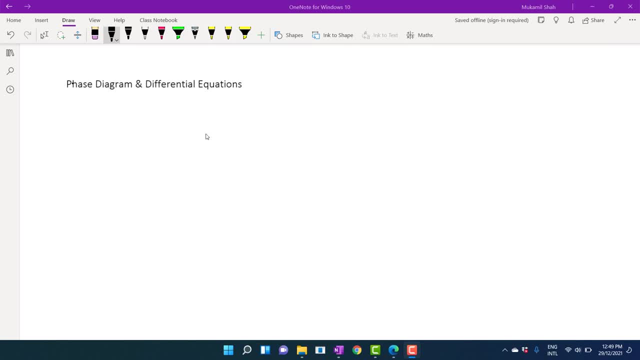 is the function of t. So phase diagram is the only tool which can help us to get qualitative information about the differential equation, whether they are converging to the steady state position over time or not. So what is the mechanism of phase diagram? what is the framework of phase diagram? how can we? 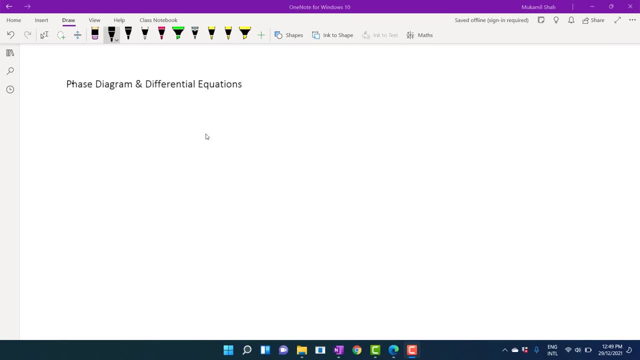 use to use phase diagram to analyze the long-run equilibrium differential equation. To understand this, let us take an example. So this is the example for which we want to draw the phase diagram. In phase diagram, we actually analyze the moment of this Y dot. What is this? 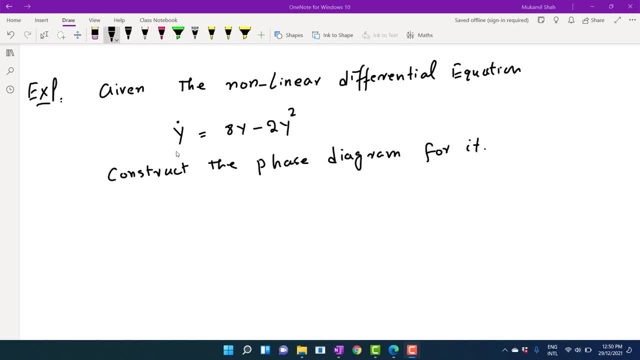 Y dot. This is the time derivative of the variable Y. In phase diagram we normally sketch two panel diagramthat is, which contain x axis and y axis, And we will observe how this y dot moves and how it intersects this horizontal axis. In the horizontal axis we take y and on the vertical axis we take y dot. We will 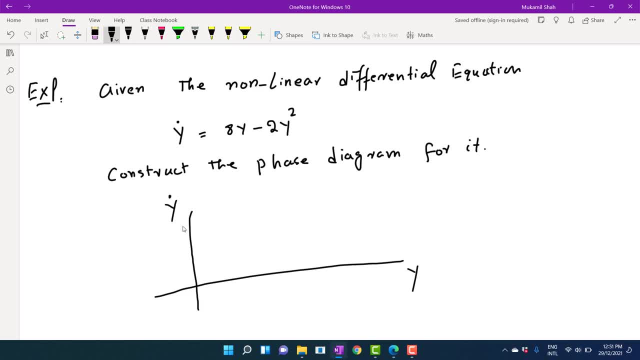 observe the movement of this y dot and we will extract information from it. First of all, we have to clarify the points at which this y dot will intersect this horizontal axis. So we have to identify those points at which this y dot this time derivative. 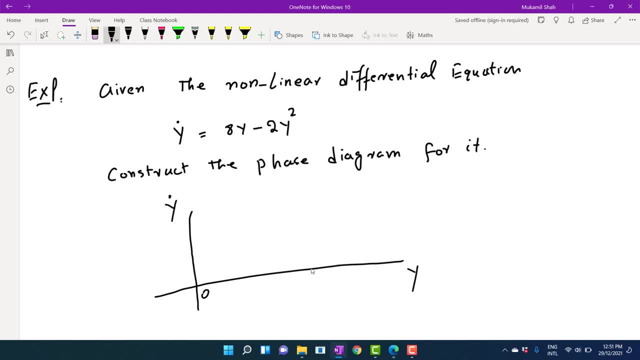 of y will intersect the horizontal axis. How can we identify those points? We can simply put this y dot equal to 0 and we will identify those points. For example, y dot, this is equal to 8y minus 2y square and you can put it equal to 0.. Solving. 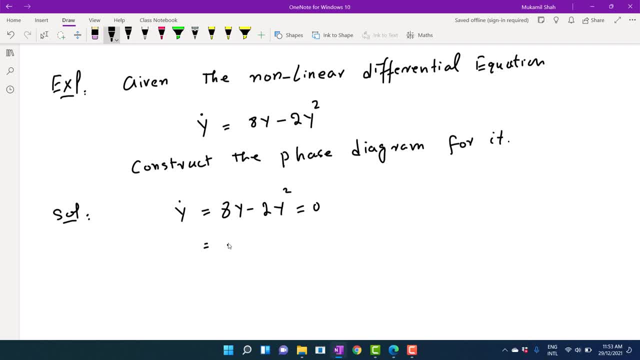 for y. so if you take something common, for example, if you take 2y common, this is 4 minus y and this is equal to 0. This implies y is equal to 0 and y is equal to 4.. These 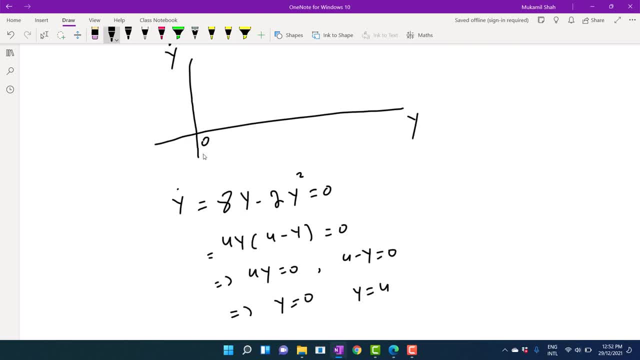 are the steady state solution. So these are the points at which this y dot intersects. the horizontal axis is 0 and 4.. So the points are identified. The one first is 0 and the second is 4.. So these are the. 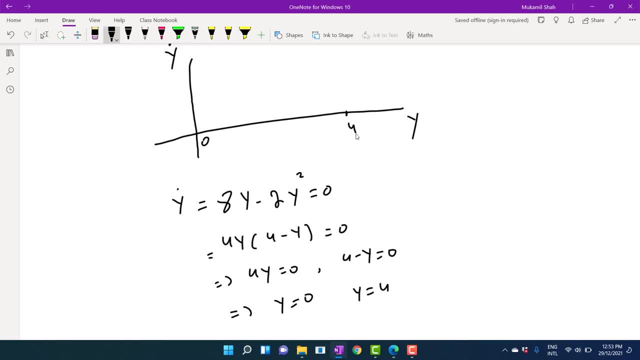 points. Now, again, there is an ambiguity: How would we draw the moment of y dot? because it can be maximized like this, or it can be minimized like this. So there are two ways, ways to intersect x-axis by y-dot, That is, y-dot can go to the maximum and intersect. 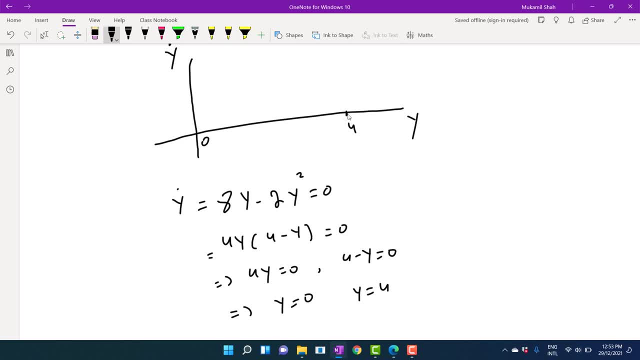 y-axis at the point 4 and 0.. The second way is y-dot can start from 0, reach its minimum and it can reach to 4 and intersect it. So there are two possibilities. We have to confirm whether y-dot would be maximized or it would be minimized. 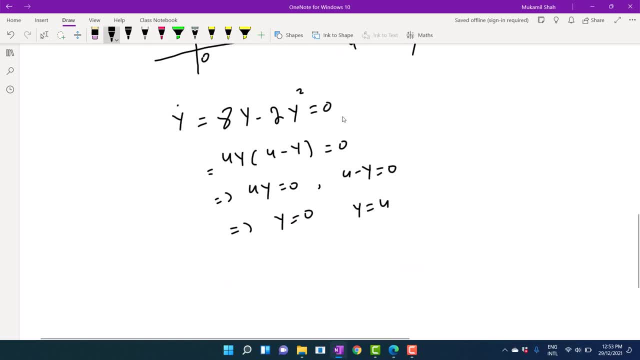 To confirm this, we have to optimize this function. We have to optimize this function to confirm maximization or minimization of this y-dot. To optimize this, we apply the first-order condition and second-order condition. First-order condition is: we take the first-order. 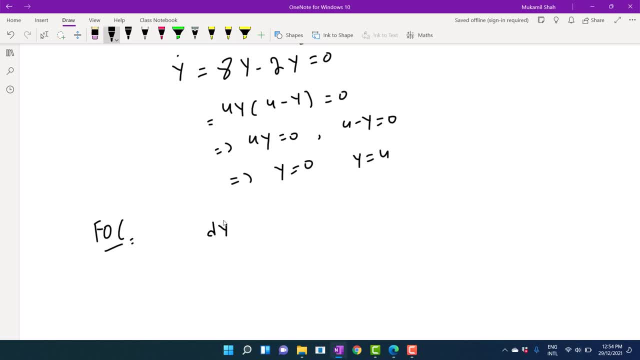 derivative of this function and put it equal to 0.. That is change in y-dot due to change in y, and this is equal to d by dy of 8y minus 2y square and we put it equal to 0. So this is 8 minus 4y and this is equal to 0. So 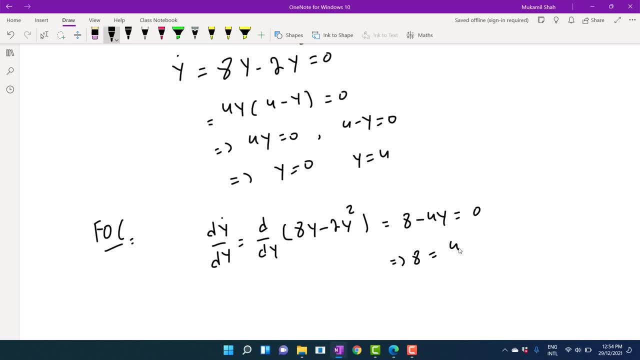 this is equal to 8.. This implies 8 is equal to 4y, or this implies y is equal to 2.. So what does this mean? It means this is the critical value, the critical value of y. If this y is equal to 2, the function. 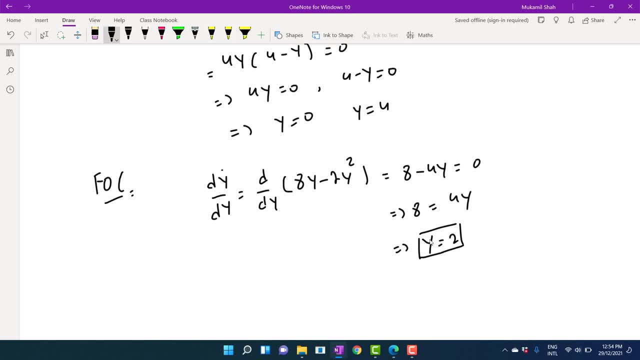 would either be maximized or minimized. To confirm this, let us take the second-order derivative, That is, we need to apply the second-order condition. The second-order condition is: we take the second-order derivative of y-dot and we put it equal to. we observe: 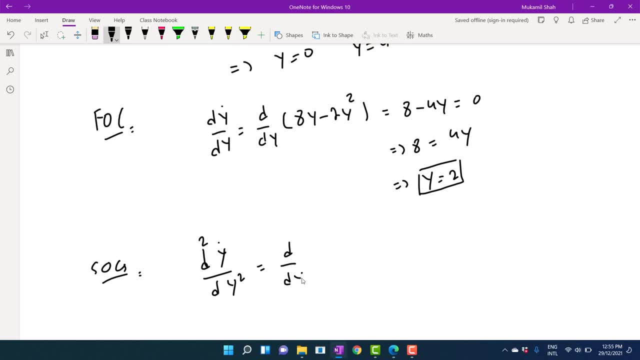 at sine. So this is equal to d by dy of the first-order condition. First-order condition is already 8 minus 4y and this is equal to minus 4, which is less than 0.. And we already know that if the second-order derivative is negative, then the function gets maximization. So the 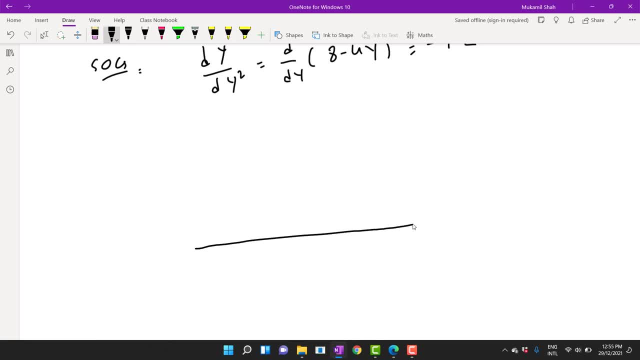 graph will be something like this: This is 0.. The graph starts from 0.. It will reach its maximum and it would intersect the y-axis at 0.. One point is this one. The second point is this: This is equal to 4.. All right, And 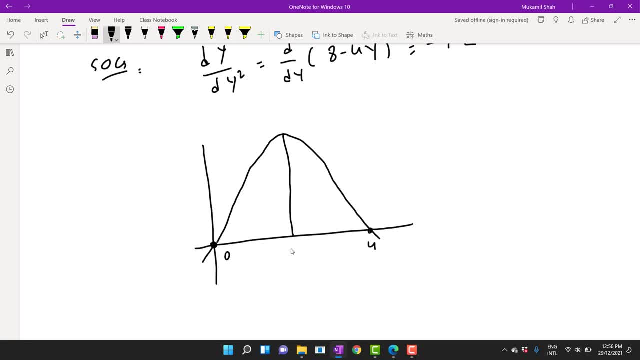 this is the maximum point. This is the critical value, at which y is equal to 2.. So that is why we sketch the graph of y-dot this way, because it is getting maximized. Here we put y and here we put y-dot. All right, Now how? what are the rules for phase? 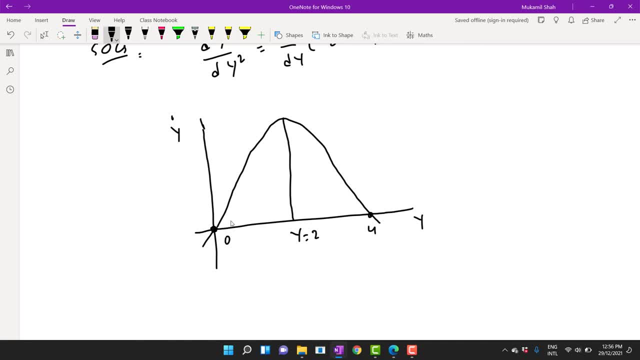 diagram. Two points must be noted. First of all, if the y-dot- this is the y-dot graph- if it lies above, if it lies above the horizontal axis, it will move to the right-hand side. So, at this point, it will move to the left-hand side. So, at this point, it will move to the. 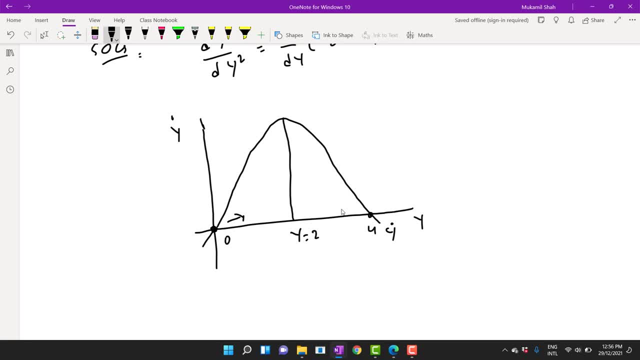 right-hand side And it should move to the right-hand side. Similarly, it should move to the right-hand side at this point as well, because above these points, the y-dot lies above the horizontal axis. Now look at this: Below the horizontal axis, y-dot should move. 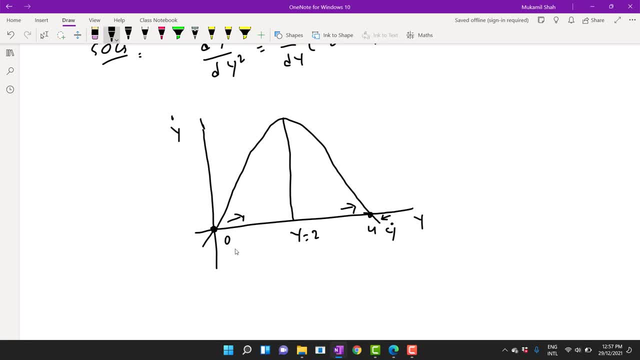 to the left. So that is why its direction should be to the left and its direction should also be to the left. Now look at it. Observe the arrow of motion directions. Observe the direction of these arrows of motion. If they are deviating from each other, then solution will be unstable.